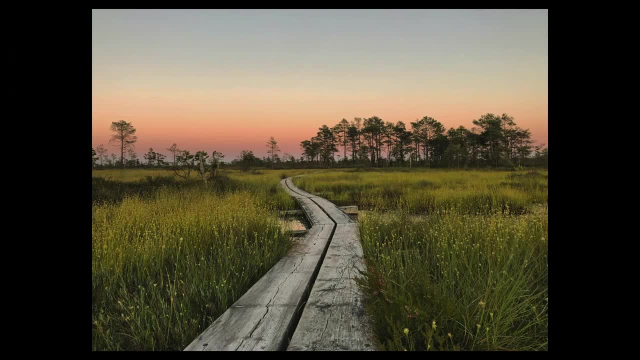 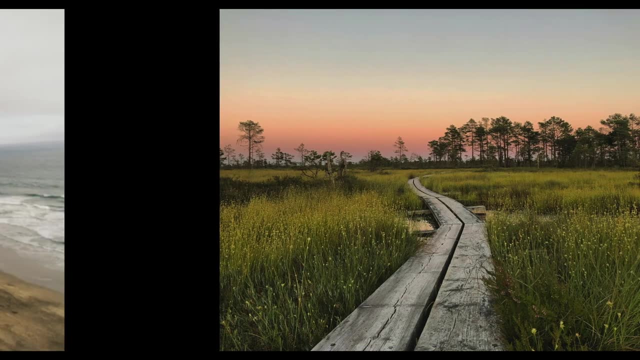 of a rule of thirds. How about the use of a rule of thirds? How about the use of a rule of thirds? How about the use of lines in photographs? How well do you do that? Are the lines complete in your photo or are they cut off? Does this help or hinder the composition? A frame within a frame is 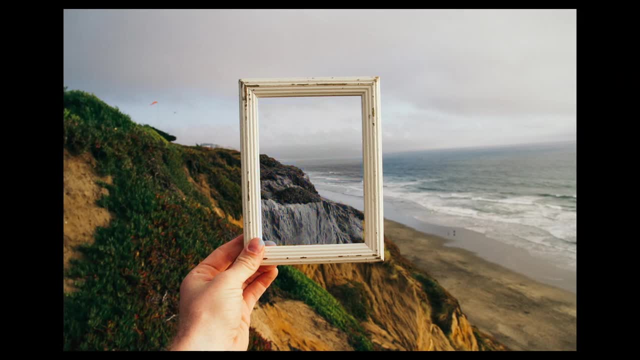 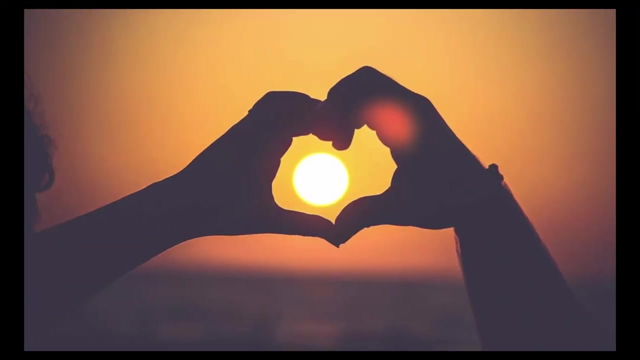 another popular rule of composition that is sometimes not used as well as it could be. When you've applied this rule, look at your photographs and see if it really works the way you wanted it to, or if you could improve on it the next time, Analyzing your photo to see how. 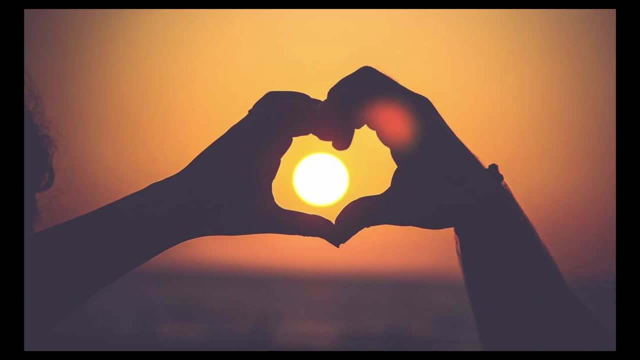 well you've framed your subjects within a frame can help you see if it worked well that time or what you could do to make better use of the same technique next time you find a frame. to put your subjects in Negative space within an image must also be considered. 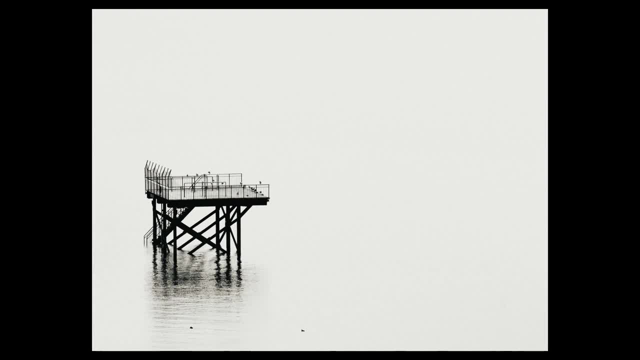 when you analyze the photograph, Does the space work to enhance your subject or does it make the image somewhat unbalanced and odd looking? You've got to make sure when you use negative space, that it's very intentional and works to enhance and improve the photograph. 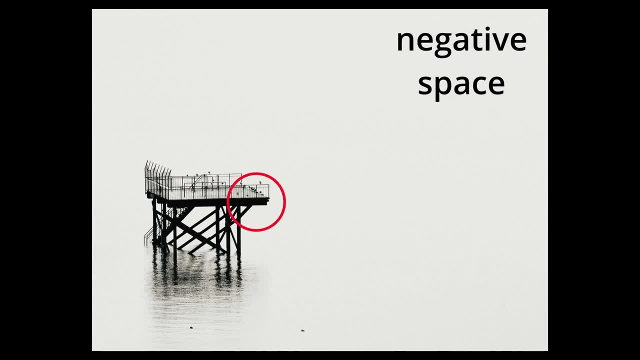 And analyzing an image based on only the objects or elements in the image and not considering the negative space is going to miss out on a lot of potential. You must think about the elements, the objects in an image, the people, if there are any, and how these things relate to the negative. 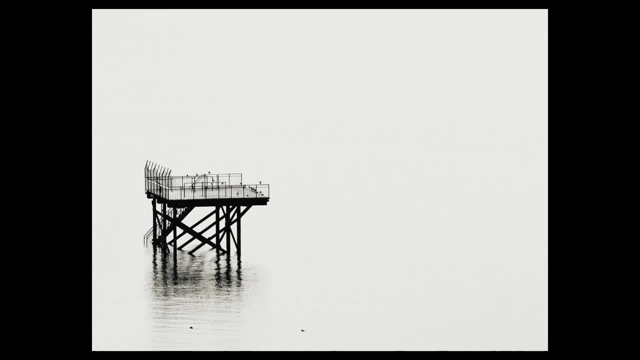 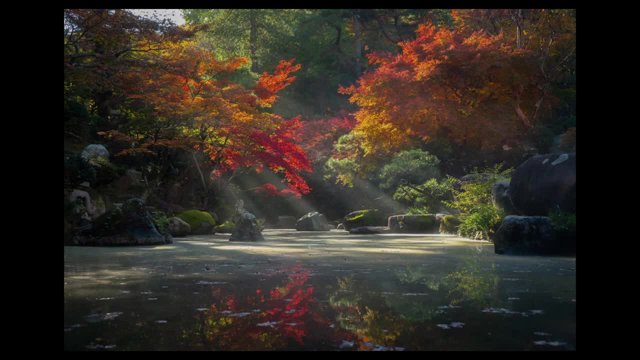 space. You must determine the relationship between these things and when you can consider this, when you can see if there is a symmetry, if there's a connection, if there's a relationship between these things, then it will either help you to see whether it's worked or whether maybe there. 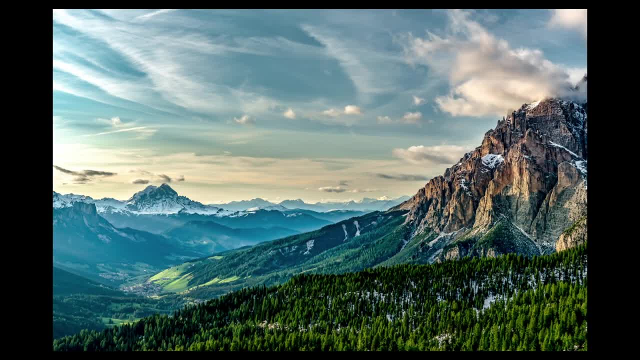 is some need for improvement. But if you're not looking carefully at the photos you've already made, you could just make the same mistake over and again and not really understand why you're not so happy with your photographs. It's also important to look at your photographs and analyze how good 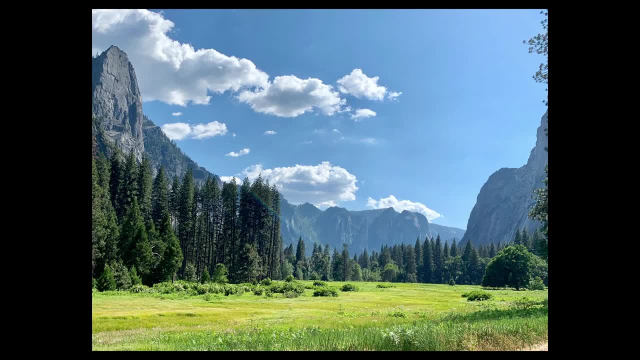 your timing was. It's important to look at your photographs and analyze how good your timing was. Did you take the photograph at the best moment or would it have been better to wait a little bit longer or have pressed the shutter button earlier than you did? Timing makes the most difference in